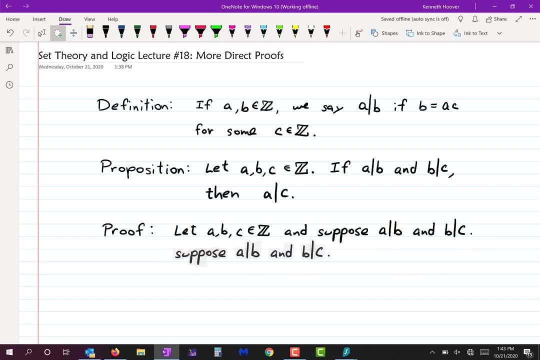 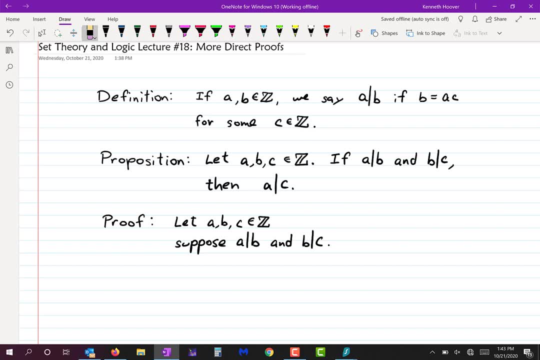 Okay, so let's start out at the beginning. Imagine a capital S on the word SUPPOSE. Okay, I could have done that, But this is all part of the hypotheses, So it makes sense to me to put them in one line. 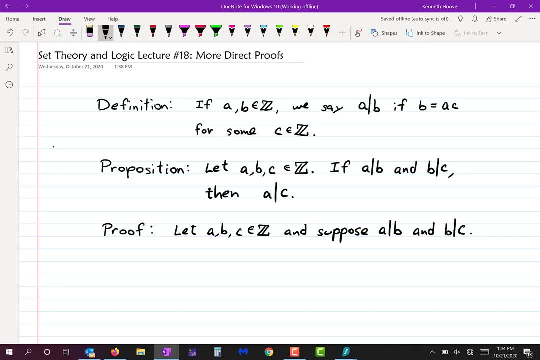 It's up to you though. Okay, Now, that's where I'm starting with, That's what I'm given, What I want to prove, I want to prove A divide C. So my goal is to work my way down and to be able to say, therefore, A divide C. 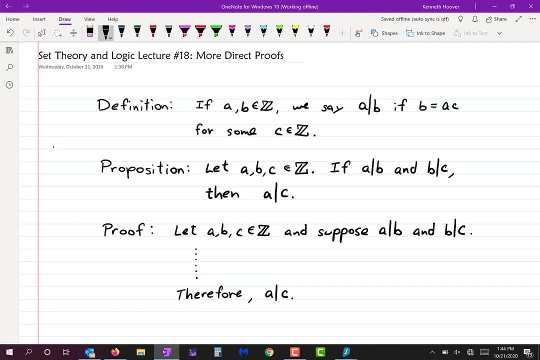 Okay, and we'll give a reasoning for that when we get there. Okay, now how am I going to show that A divide C? Well, the only thing I have to go by is the definition of divides. So I'm going to show that A divide C by showing that C equals A times an integer. 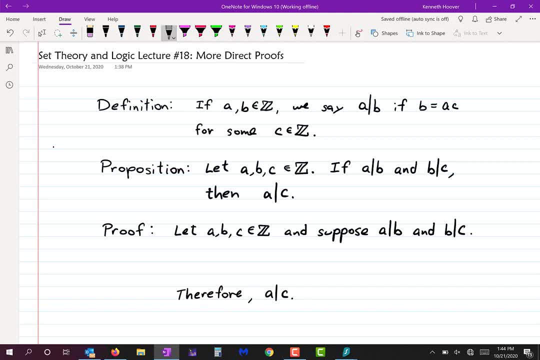 Do you agree with that? The penultimate line, which means the one before the last, is going to be saying that C equals A times an integer. Do you agree that? that's what I need to get to? And then, once I get there, then this will be automatic. 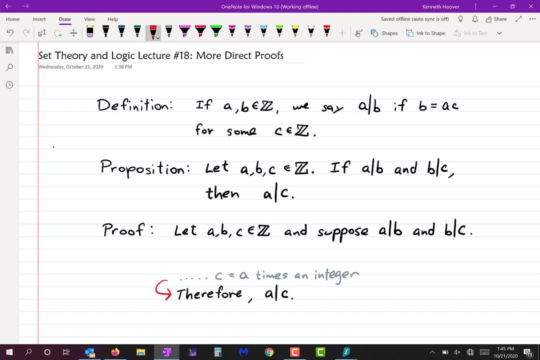 I'll be able to say A divide C, Because I will have shown that A fits the definition of dividing C. Okay, so how am I going to get to? C equals A times an integer. Let me write it like this: A times integer. 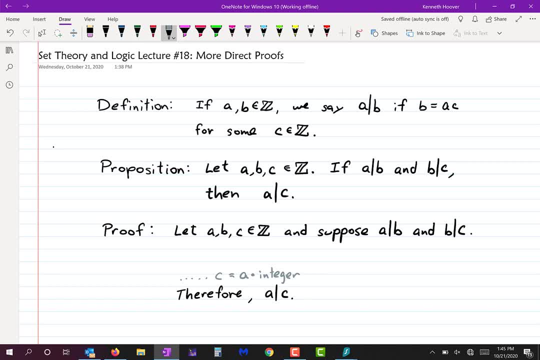 How am I going to do that? Well, let's go back to the top and try working our way down towards that. Okay, what do I have to work with? Okay, Okay, Okay. So I have that A divides B and I also have that B divides C. 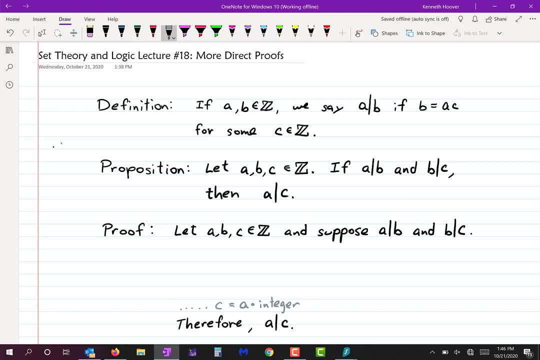 And I know what it means for one number to divide another right. So since we have A divides B, let's write down what that gives us. Okay, so then what's that mean? It means that B equals A times some integer. 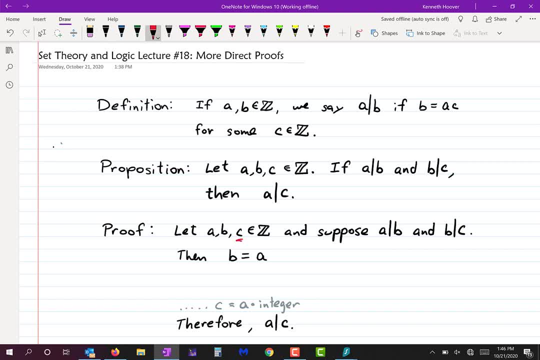 Now, I can't use C here, because C is being used for something else already. So pick another letter. How about we'll just go with D? Okay so, because A divides B, then B equals A. Whoops D for some integer D. 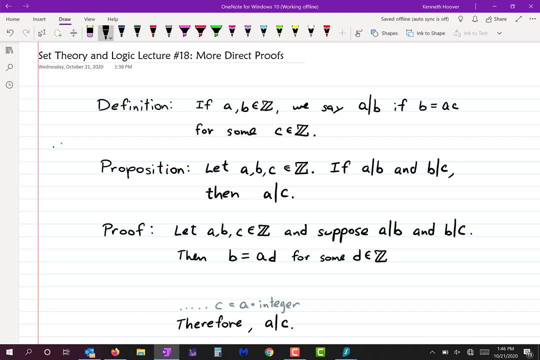 Okay, and we might as well go ahead and say as well that: what does C equal? C equals B times some integer right? What do you want to call it? You want to call it E, E. And what is my reasoning for saying that? 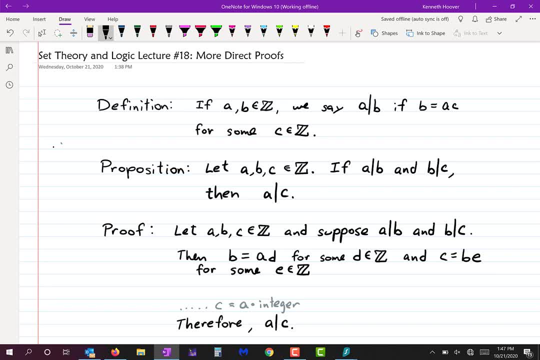 Because A divides B and B divides C, And that's what the word D is, Divides means. So I'm going to write by the definition of divides. Okay, Okay, All right, Now you've got to be a little bit creative here. 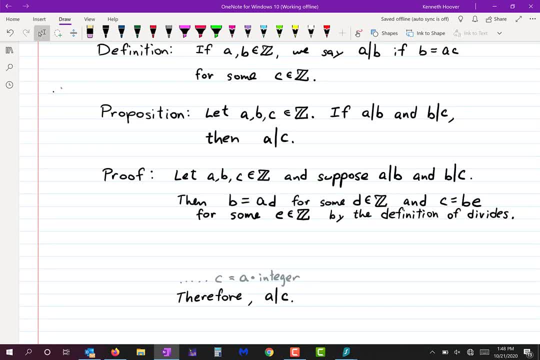 You can't just, you can't always just follow, Follow the breadcrumbs without thinking of where you're going, because there's almost never enough breadcrumbs to lead you all the way. So you have to be also creative And you've got to think about how am I going to get from point A to point B? 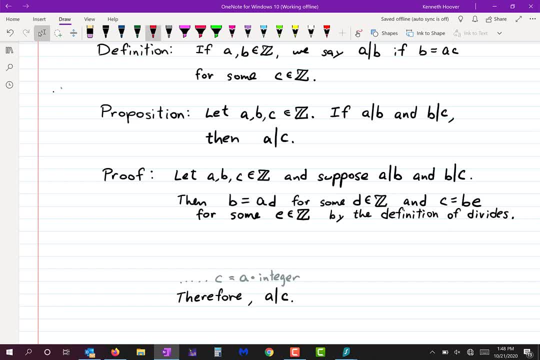 Okay, So how are we going to get from where we just left off down to here? It's not a difficult guess to make. What do I know? I know that C equals B times E, And also I know that B equals A times D. 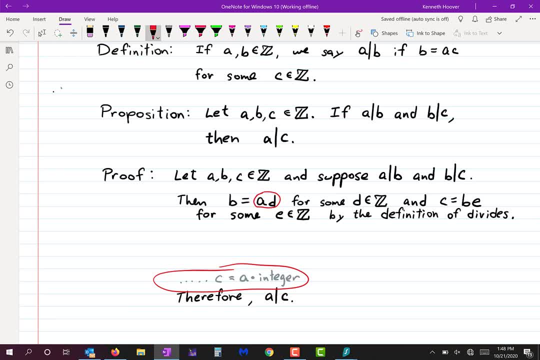 So can't I just take that and substitute it in for B, right there? And then what will I have? I'll have C equals A times D times E, Correct, Correct. So Let's say: hence: C equals. So I'm going to substitute AD in place of B. 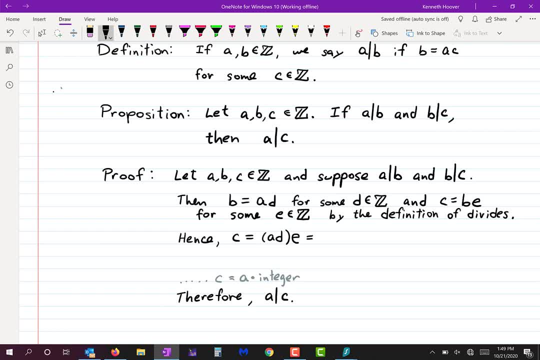 And then I'm going to use the associative property to write that, as instead of AD times E, I'm going to write A times DE. Isn't that exactly what I was wanting? I just have to point out what I have to point out something about this. 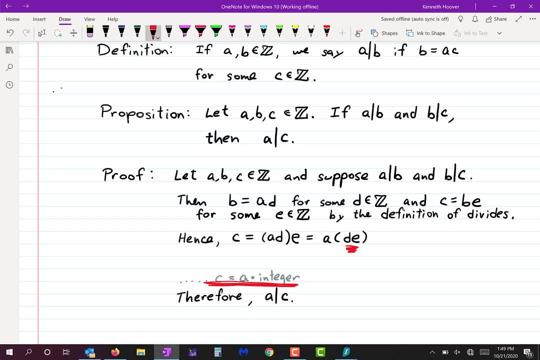 In order for me to be finishing my proof, DE needs to be what kind of number? It needs to be an integer. Let me ask you a question: Is it an integer? Yes, it is, because D is an integer And E is an integer. 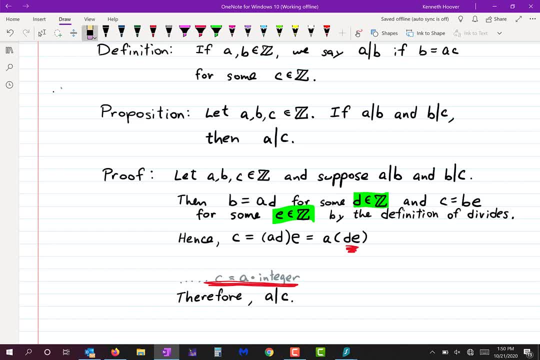 And an integer times An integer is an integer, So DE is in fact, an integer, But it's my job, though, to point that out. I can't just say, oh yeah, it is true. No, I've got to say it. 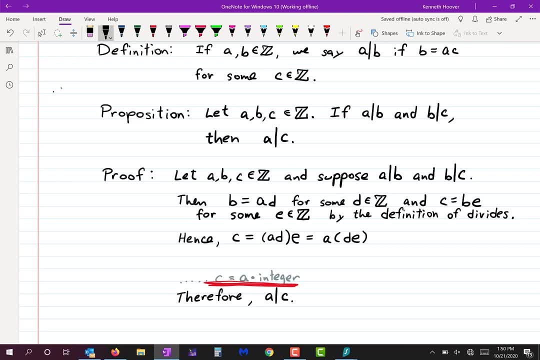 I've got to put that in writing, Okay. Okay, So I'm going to say where DE not D, comma E, but the number DE is An integer. Okay, I suppose I'm just trying to think back. That's why you're probably wondering why I paused. 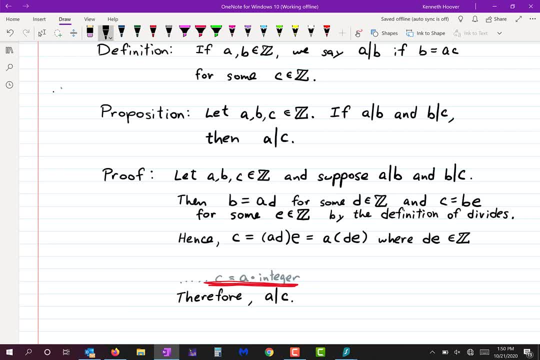 I'm trying to think back to the previous example that I did And I'm just trying to give you. I want to give you some different views here. Okay, And I could, if you don't like the way this looks. DE is an element of the integers. 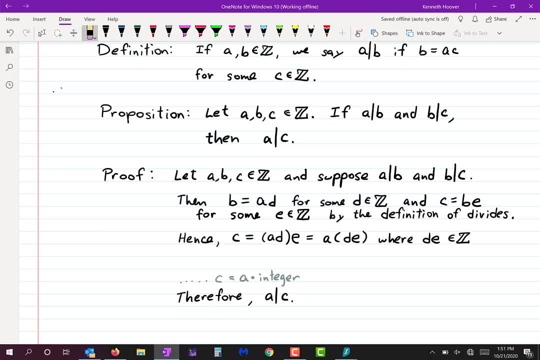 Here's what you could do: Give DE its own name. What do you want to call it? Should we call it F? So then I could say this Thus: Here I'm going to take that off of there And I can say thus: 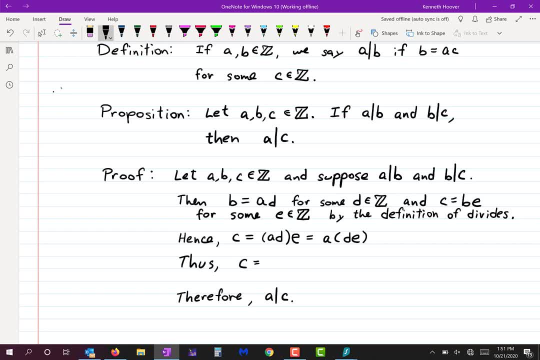 C equals AF, where F equals DE, which is an integer, If you prefer that. that's fine. Okay, And then we have our conclusion. Therefore, A divides C, And why is that? What am I basing that conclusion on? 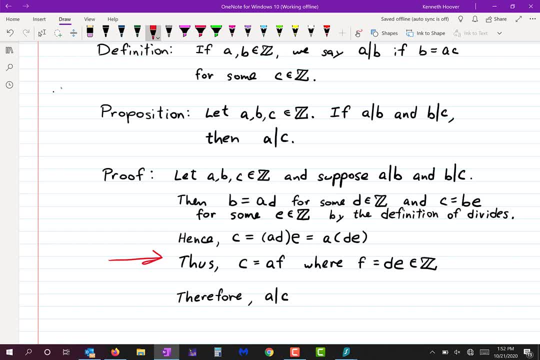 I'm basing it upon the previous line and the definition of what The definition of the word divides. Why did I not write a reasoning down for these two lines? Why did I not write a reasoning down for these two lines? Why did I not write a reasoning down for these two lines? 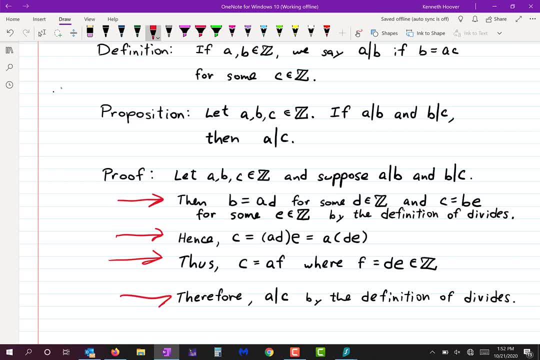 Because I wrote a reasoning down for these two. Why did I not for the two in the middle? Because what did I do in the two in the middle? I just used in this line here, I just used ninth grade algebra right. I used substitution to substitute AD in place of B. 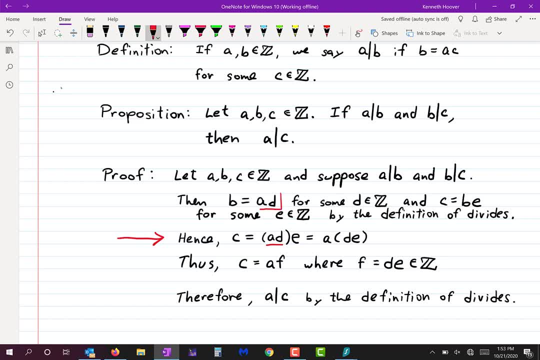 Because of this allowed me to do that, And then I used the associative property to shift to the parentheses over. That's all. You don't have to write down by substitution and the associative property. That is taking it a little bit too far, being a little bit too trivial. 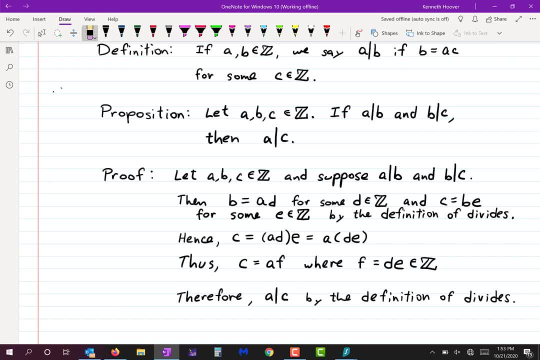 Okay, I said this last time, You don't have to verify your use of the commutative, The distributive property and the distributive property and the associative property. All that basic ninth grade algebra stuff is ninth grade algebra. Okay, You don't need to give justification for your basic algebra steps. 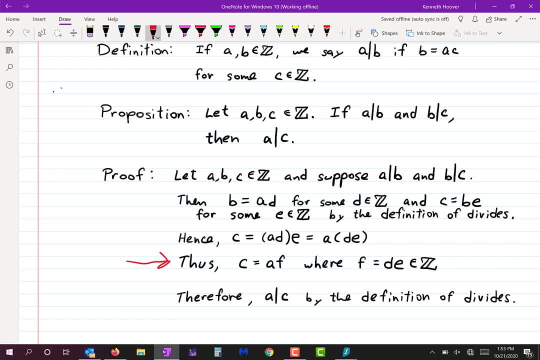 How come I didn't give a justification for this? Because I didn't really do any math here. All I did was just renamed the number And I gave it a name. that is a single letter. And besides that, remember, I told you that you don't even have to have this line if you wrote the previous line the way I did before. 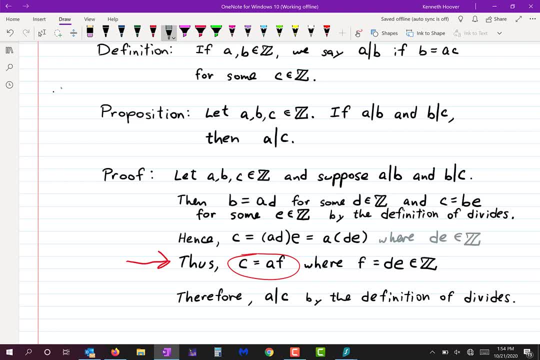 If you have this at the end of the previous line, then you don't even need the next line to be written. Okay, So what I circled there? C equals AF. That's simply giving DE a name of the single letter F. 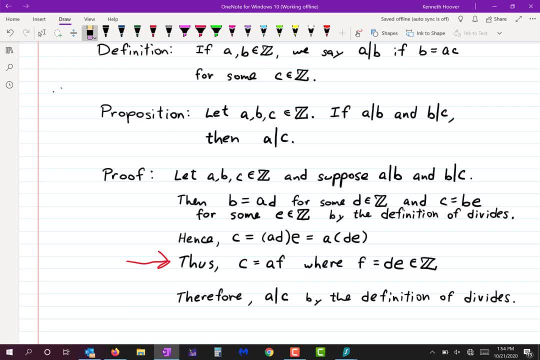 And what else have I done in that line? Pointed out that that is an integer. Okay, Why is DE an integer? Because DE and E are both integers And when you multiply two integers together, you have an integer. That's called the closure property of the integers. 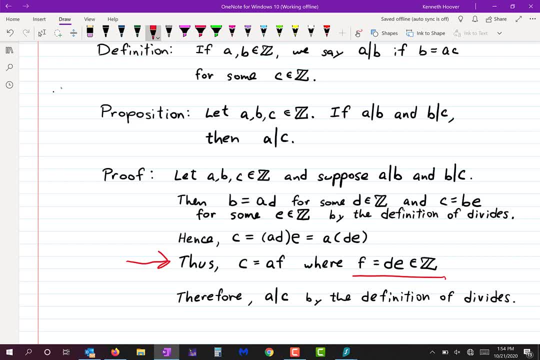 And if this was an abstract algebra class- I forgot what number that class is- Then maybe I would write that down. But I just you know, I'm just being honest with you. I don't think it's necessary to point out here that an integer times an integer is an integer. 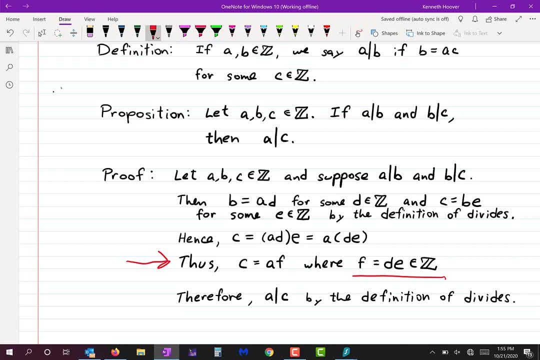 You're going to have to learn what needs to be pointed out and what does not require being pointed out, And an awful lot of that has to do with The setting. What is it that you're trying to prove And what is your audience? 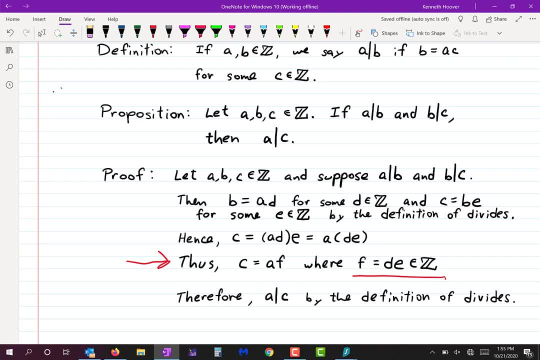 If I was trying to prove this for a ninth grade class, then I would have pointed out my use of the associative property and the substitution property. I'm not pointing it out here because you guys aren't in ninth grade. You see what I'm saying. 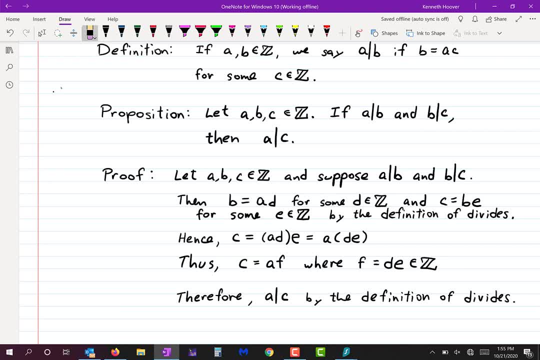 I hope that's not too vague, But These are some things that you have to get a feel for and you have to decide. It's better, if you're not sure, It's better, to give more justification and have more than you need than not enough. 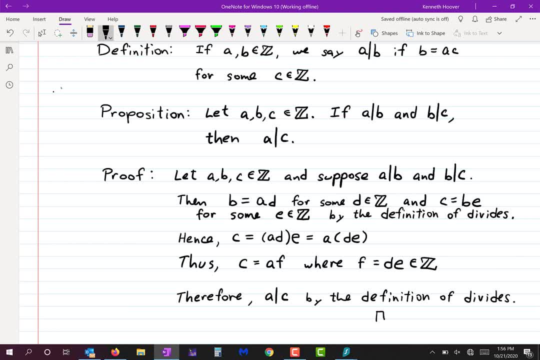 Okay, All right, let's see what's next in the book. You can see this proof in the book too, and you'll see it's almost exactly like I've done it. It's just some different words, like the word, likewise. 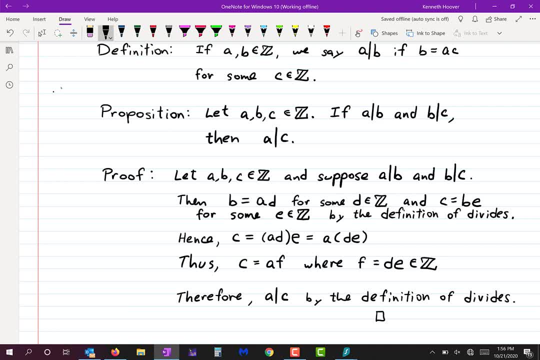 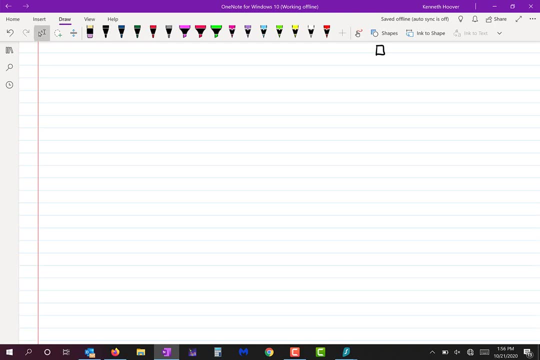 And instead of using F for D times E, they've used the letter X. That doesn't make any difference. Okay, let's do this one. You're going to have to remember the definition of even and odd, So if you don't remember that, look at the last lecture and look that up. 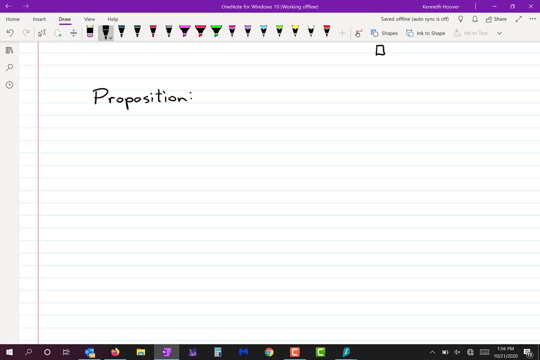 Okay, If X is an even integer then, By the way, before I go any further, just so you know, when we use the word even and odd, those words only apply to integers. So I could say, if X is even, that would be okay. 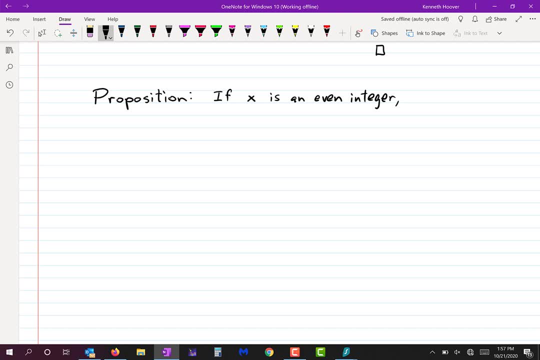 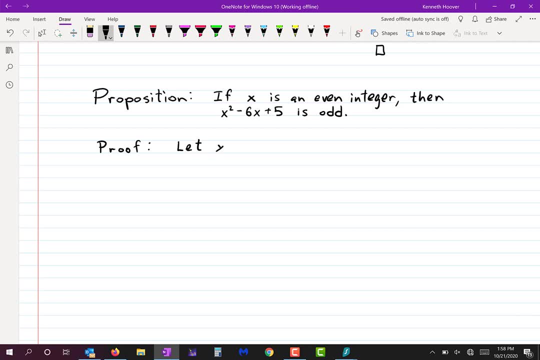 going to start with: let X be an even integer. I'm gonna write it like this: let X be an element of the integers, that's even so. we write it like this. I know if I said that in words it would sound odd. I would say: let X be an. 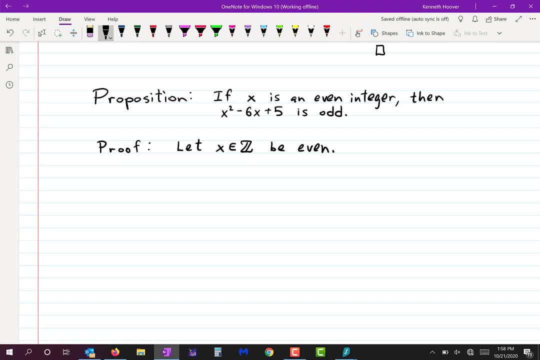 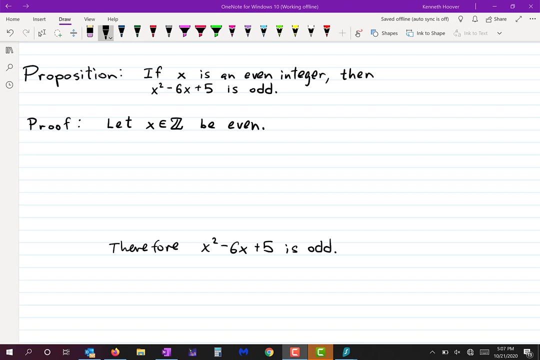 element of the integers be even. I know that's not grammatically correct, but when you write it down, that is the the way you would normally write it, because I can justify that by saying like this: let X in the integers be even. that's how I would say it to make it sound grammatically correct. okay, now we. 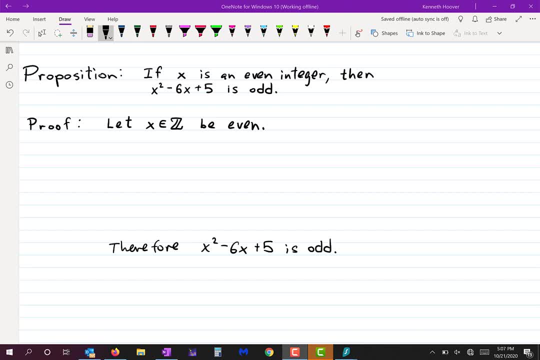 need to figure out how to get from that first line to the last line. right, let's take one step in each direction. from the top, we'll take a step down, because X is even. what do I know about X? I know that it fits the definition of even, which is: 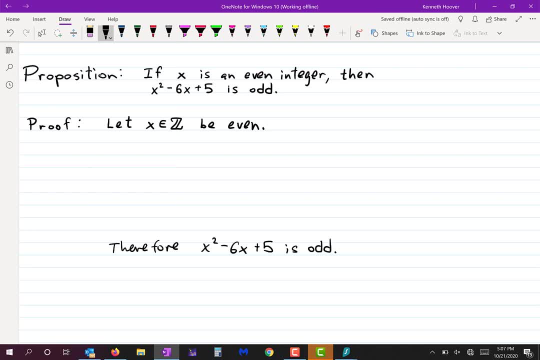 what two times some integer? okay, so I'm gonna write: then: X equals two times something where that something is an integer. and why do I know that? I know that by the definition of even. okay, let's go to the bottom and take one step up. what would allow me to? 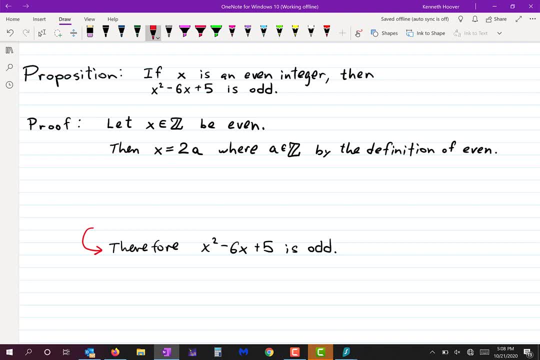 conclude that X is odd. I can conclude X is odd if X fits the definition of odd. what's the definition of odd? a number that is two times an integer plus one. so my goal is to get to this point, then X squared. I may have said X a minute ago. 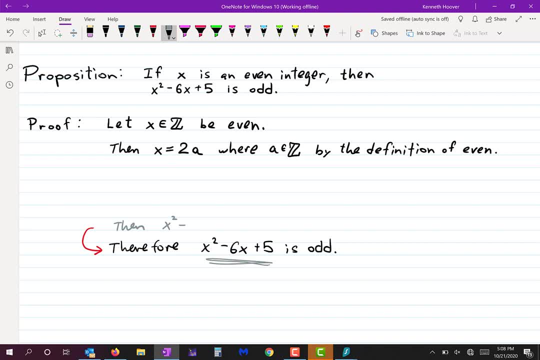 and I didn't mean X, I meant this number that's there, which is X squared minus 6, X plus 5 equals. hopefully, we'll be able to show that it equals X squared minus 5. so that's the definition of even. okay, now let's go to the next definition. what would allow me to? 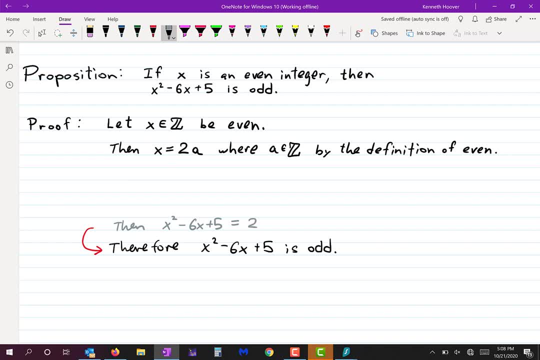 predict the whole thing to be even so. we're gonna just write it down like this: we'll be able to show that it equals two times something plus one where that something is an integer. now, i'm not writing that in gray because i know this not at all. it's exactly the other way. 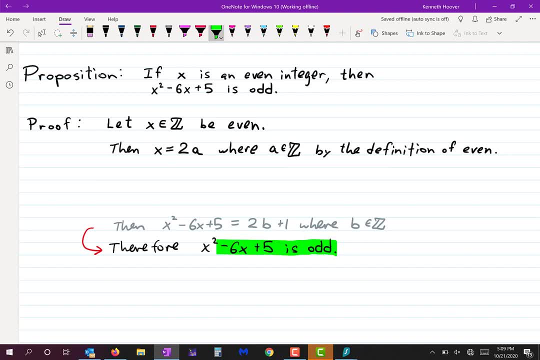 around. i want to know this and i will know that if i can get to here, because then i can say that that number is odd by the definition of odd, and then i'll be done with my proof. so the question now becomes: i don't have to worry about this anymore. 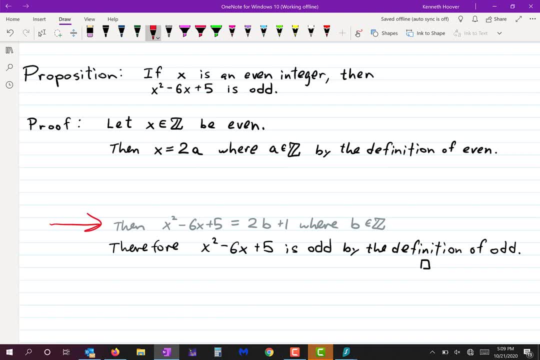 now i just have to try to get here and technically you could start at the end of a proof and work your way all the way back to the beginning. i personally like to do this. i like to take maybe one step back from the end, just so that i have an idea. 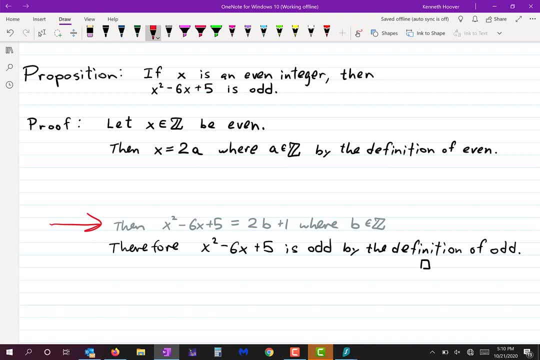 of what i'm trying to get to and the rest of my work. i like to go from from the beginning and move forward. some people like to do the same amount of work in each direction and meet right in the middle. you know i usually do about 80. well, i at least think at the beginning, i at least 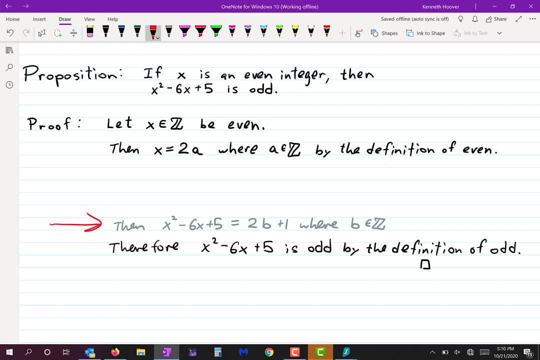 think about what does my penultimate line need to be? penultimate means, uh, next to last line. i think to myself: what does my next to last line need to be? maybe i don't write it down, but i at least think about that, so that i have for myself a mental goal. and then i go to the front. 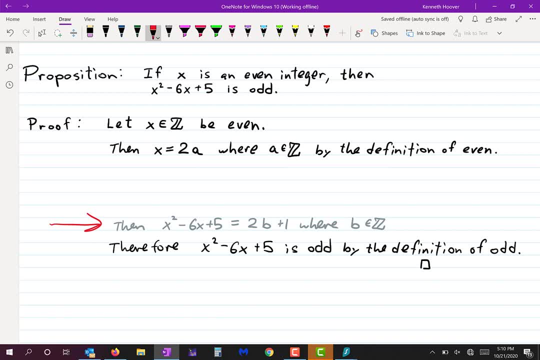 and try to work my way to that. if i can't figure out how to get there, then i go to that penultimate line and i try to figure out, okay, well, what will need to come right before that, you see, okay, so, anyways, let's go now to where we left off there on line two. 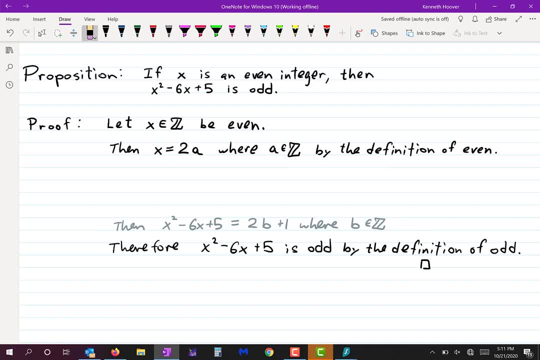 and let's figure out where line three is going to come from. okay, so i don't know anything else about x. it's an integer that equals two times an integer. that's all i know. so at this point i'm thinking about: okay, i should probably now 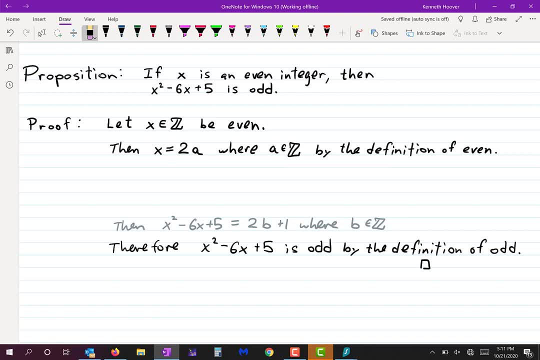 start transitioning. i can't say anything else about x, so i should probably start transitioning to the number that they're actually asking me about, which is that number. okay, well, i can do that right, because if x is 2a, then i can say something very important about x squared minus 6x plus 5. 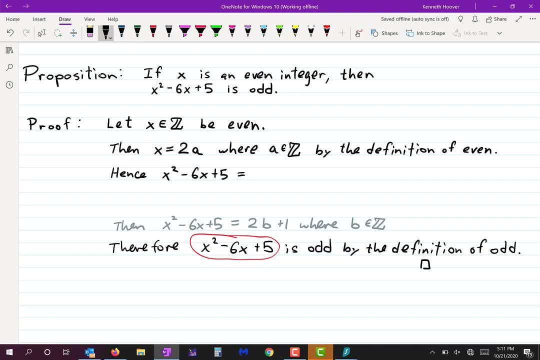 can't, i can't. i say what that would be. it would be 2a squared minus 6 times 2a plus 5, right? i just used the substitution property there. this allows me to change this into this. okay, now let's simplify that. what does that equal? 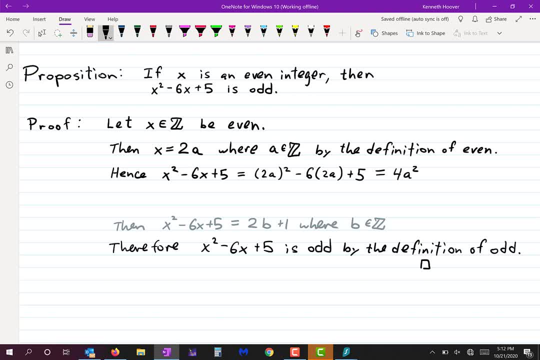 wouldn't that be 4 a squared minus 12 a plus 5.. now let's talk about what should you show versus what do you not need to show? you might be asking this question. you might say: could we have just said this, could we have just said that? and the answer is yes, you could have. 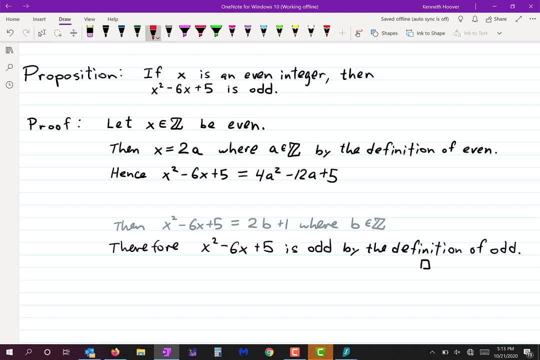 i personally think, if you do that, if you go straight from here to here, i think that's too big of a leap. not that it might not be true, but here's the, here's the overriding principle. okay, remember- i don't remember if i said this earlier in this lecture or not, but remember that when laws 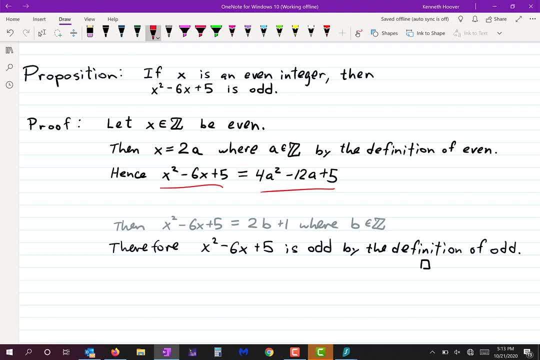 are written in the laws. it always says, or usually says a reasonable person: okay, if you use violence to defend yourself against somebody, are you going to go to jail for that or not? they are going to ask themselves in court. would a reasonable person have been in fear for their? 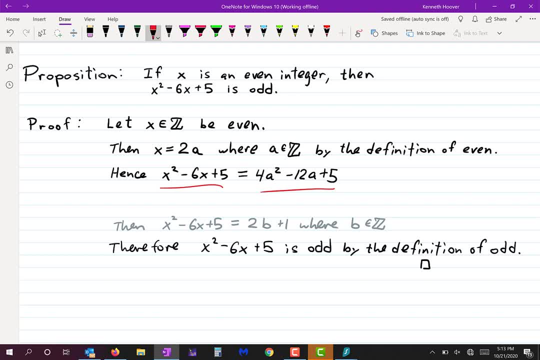 life, and if so, then you probably won't go to jail. so when you're writing your proof, you have to ask yourself: would a reasonable person see what i wrote and have no questions? that's what you want to ask yourself. now, i think, to go from here. 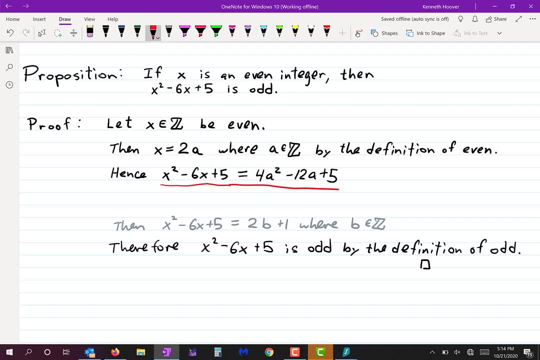 to here. i think a reasonable person would have to stop and say, okay, what did they do there? i got to figure this out, and if and if somebody has to stop and say that, then that means you haven't shown enough. okay, now somebody who's not good at math might have to stop and think you don't want to. 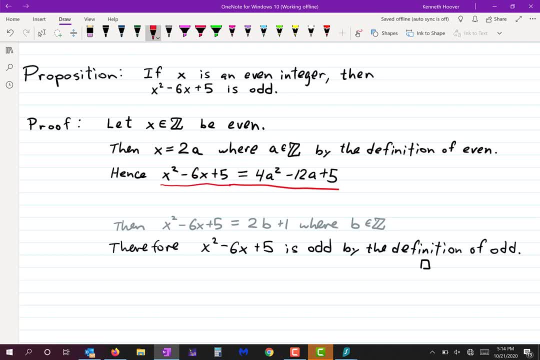 worry about those people. you want to worry about someone who is at the level that they can follow this mathematics. okay, they might have to stop for a second here or there, but if they have to stop and really think where did that line come from, then that means you haven't shown enough. 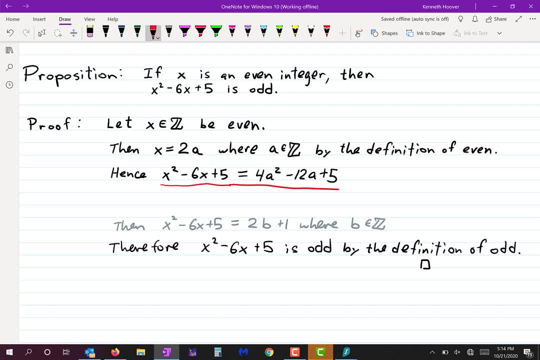 justification- and i think what i have underlined there in red, i think is- is: i think that you need that extra bit in the middle, so let's put that back where it was. you see, now there should be no question at all what's happening to anybody, any reasonable person. 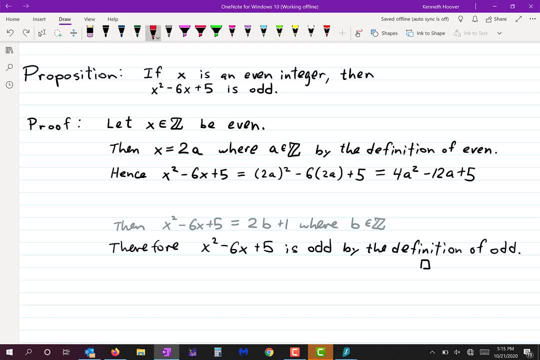 can look at that and say, oh, i see exactly what they did. they started with this. they replaced x with 2a, and then they simplified and this is what they came out with. okay, now, what's our goal? our goal is to make it look like this: 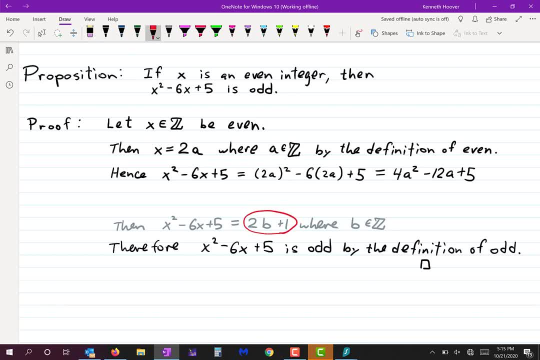 two times an integer plus one. so let's look at where we left off of there. can you figure out how i can rewrite that so that it says two times something plus one? how about this? it certainly equals 4a squared minus 12, a plus four plus one, right? 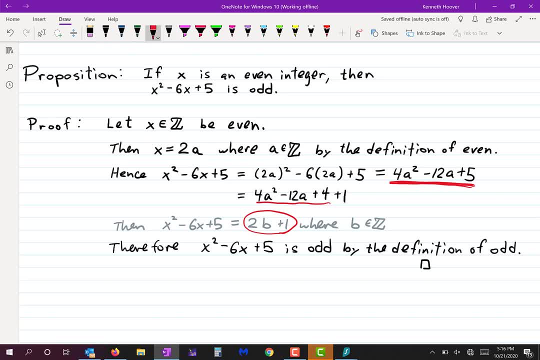 and can't. i factor out a two from here and i think that's fine to go ahead and do that here. that's not too big of a step. so we're pulling a one away from the five to get the five as four plus one, and we're going to factor out a two from those first three terms. that is, that is not too much to. 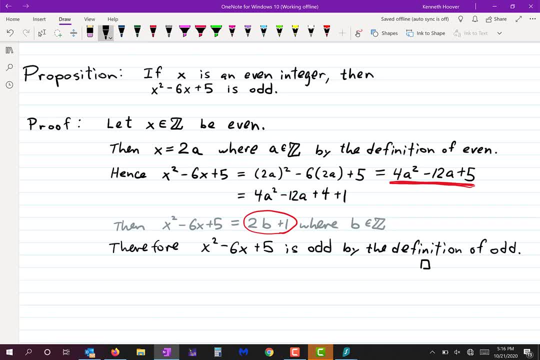 do both of those in one step. so what would it be here? it would be two times two a squared minus six a plus two. okay, so let me write that down: two times two a squared minus six a plus two, close parentheses: okay, well, now we can change that. 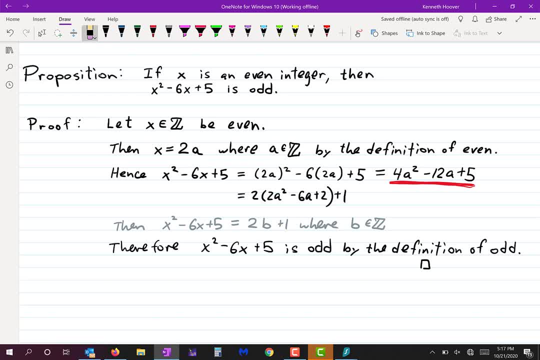 gray line to black. we. i mean, i need to change one small thing, but we basically got it. i wonder if i can just change the color without rewriting it. i'll be darn, look at that, what a fascinating modern age we live in. okay, i do need to. 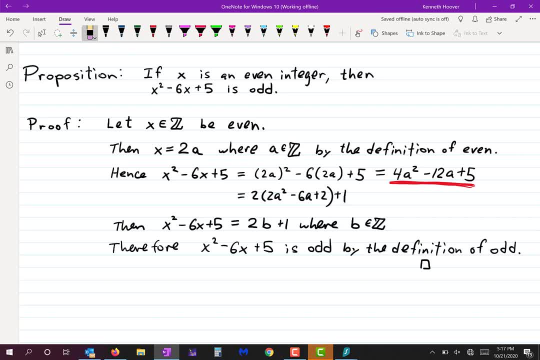 point something out, though. right, all of a sudden, this b shows up. where'd b come from? you guys know? right, i've taken this number and i've just named it b, that's all. so what do i need to do? i need to make that clear. so i just said here where b is an integer. what i should really say now is: i should really say: 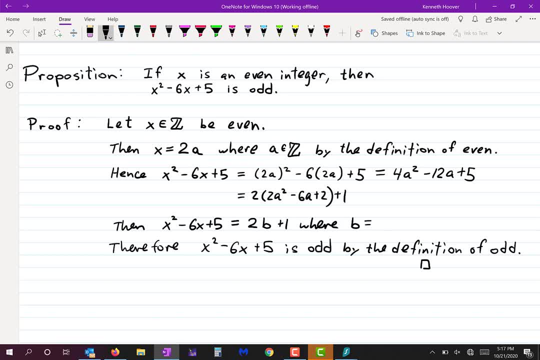 where b equals 2, a squared minus 6, a plus 2, which is an integer, and there we go, done with the proof. okay, now I do want to point something out. this is a pet peeve of mine when students do this part wrong. I mentioned this in the last lecture too, so I'm glad it came up here so I can. 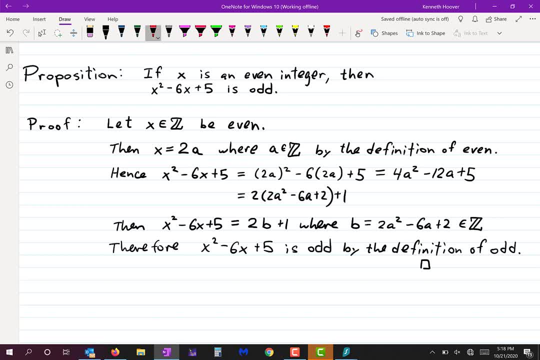 mention it again, this is not two lines. let's number the lines: number one, number two. if you did this, three, four, five, six- your numbering is not correct. if you do that, there is not six lines in this proof, there's only five lines, because that thing that I circled in red is one. 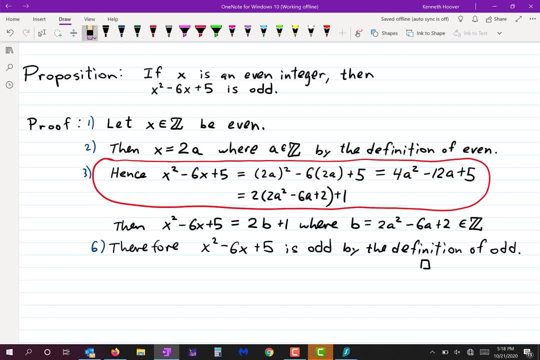 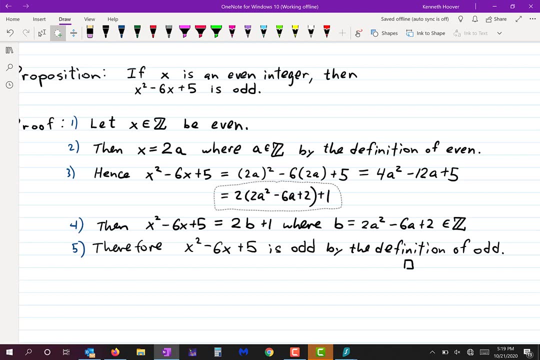 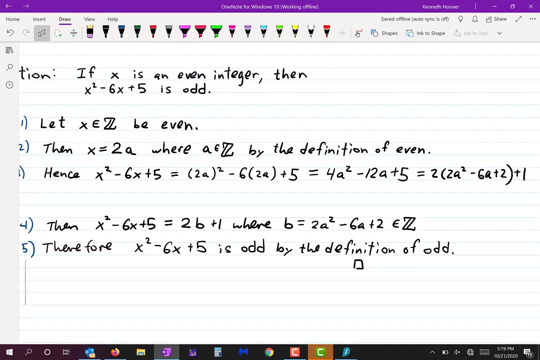 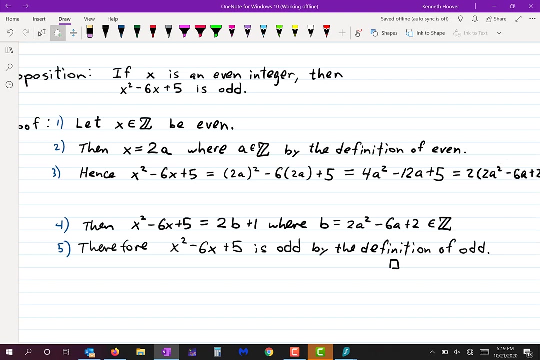 line, that is the line number three. okay, you see, this actually belongs right there. it's one line. it's just that the line was getting too long and I was running out of room, so I took that bit kind of like, kind of like hyphenating a word in a way. oh, there we go, and I just moved it down there. oh you. 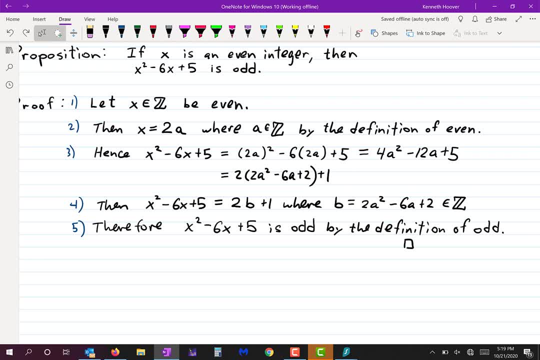 might ask this question: why way over there? why didn't I put it right there? I know the answer is zero and in fact a lot of people do. this is just a personal thing for me. I just think it looks nice to have the equal sign lined up with the first equal sign from above. it that's. 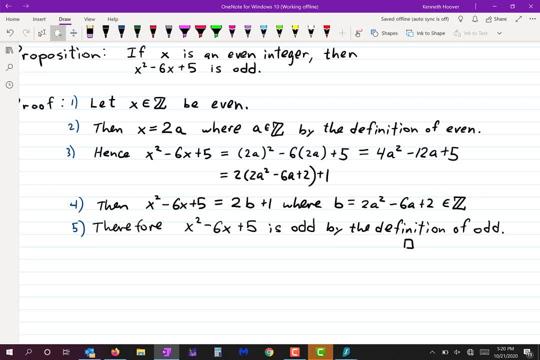 all that was personal preference. it actually doesn't matter where you put that. I could have put it over here and lined it up with that equal sign, or I could have said this: I'm going to put a line over there here and nowadays just put a line up to that side where you put your line. 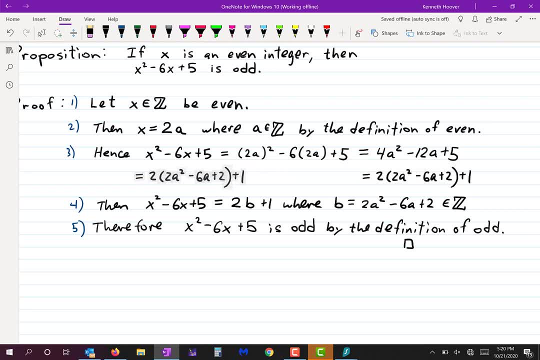 put it at the beginning. here's what I do a lot. this is another thing I like to do. you can say, okay, I'm gonna put the beginning, but visually I would like it to be obvious that this is not a new line. a new line, it is a continuation of the line above it, and so I do this a lot. I indent. 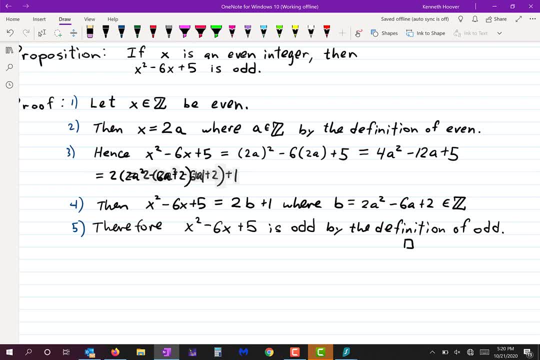 like that. that makes it clear. I haven't started a new line, I'm continuing a line. okay, now let's read that out loud. it says- I'll highlight as we go: it says: hence: the x squared minus six, x plus five equals two a squared minus six times two a plus five. 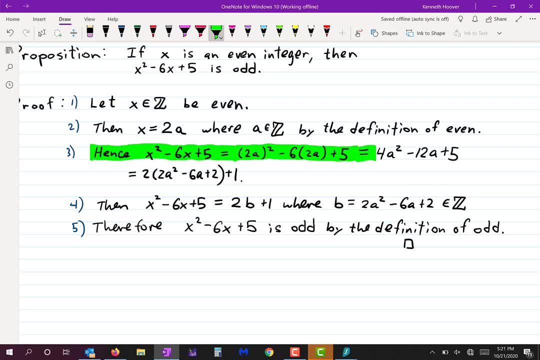 which equals four a squared minus 12. a plus five, which equals two times the quantity two a squared minus six. a plus two plus one. that's the correct way to read that. okay, that is really a smart way of condensing three lines into one. let me circle this again. what? 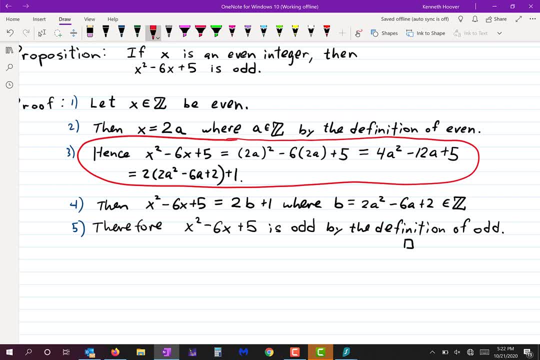 that really is. well, it's three equations, right. why am I saying three equations? because I see three equal signs. each equal sign. each equal sign indicates an equation. what I've really done there. this is important for you guys to get. if you understand this stuff now, it'll just make life so much easier on you later. what I've really done there is: I've really said. 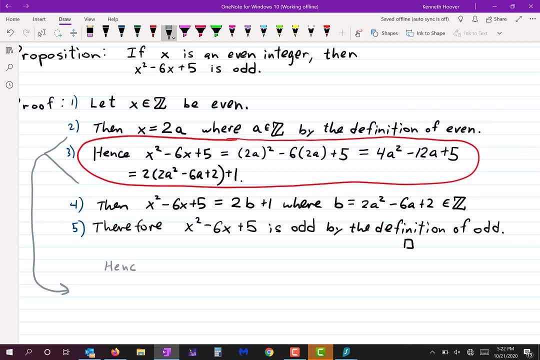 this. hence: x squared minus six, x plus five equals two. a squared minus six times two. a plus, these are the equals to two a squared minus six times two. x is two equal to five. this equation is mental: 6 times 2a plus 5.. 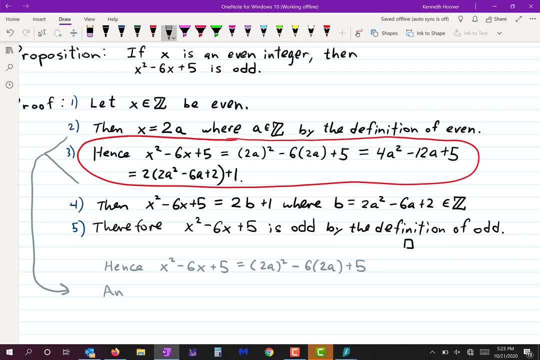 And I know you're not supposed to start a sentence with the word and, but I think that's a rule that we've kind of thrown out the window, so I don't worry about that. And 2a squared minus 6 times 2a plus 5 equals 4a squared minus 12a plus 5.. 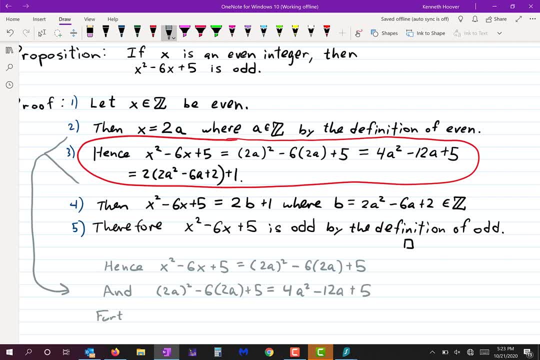 Furthermore, 4a squared minus 12a plus 5 equals 2 times the quantity 2a squared minus 6a plus 2 plus 1.. That's the three equations It could be written: 1. Equation per line. then I would have those three lines. 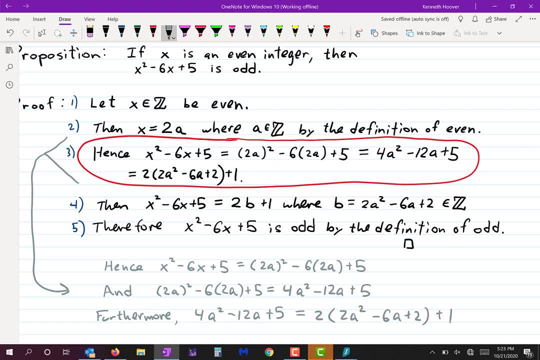 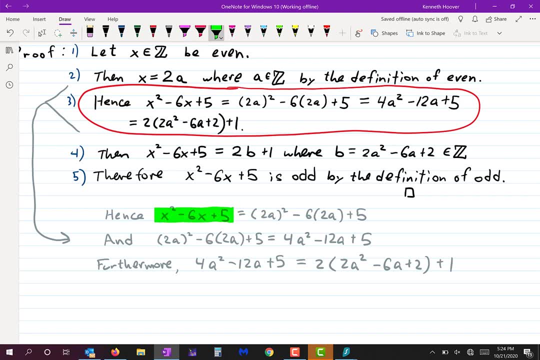 But here's the catch: If I did that, I would need a fourth line in there, because I need to show that this equals that. So I would then have to say thus: or let's say: therefore, You don't have to use therefore, only on the last line. 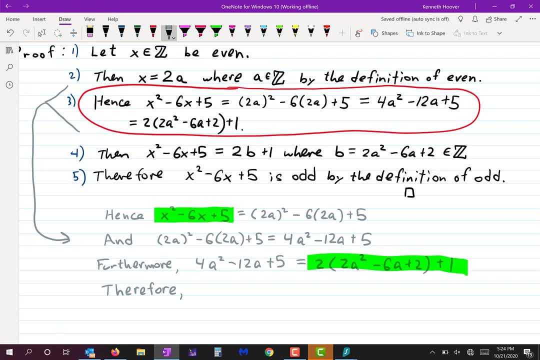 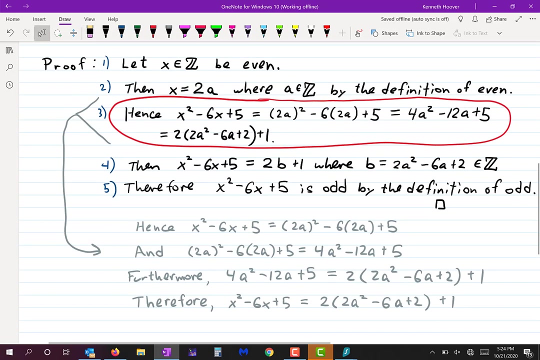 You can use it in the middle of your group too. Therefore, Therefore, x squared minus 6x plus 5 equals 2 times 2a squared minus 6a plus 2 plus 1.. Okay, So look, Those four lines have been very cleverly combined into one line. 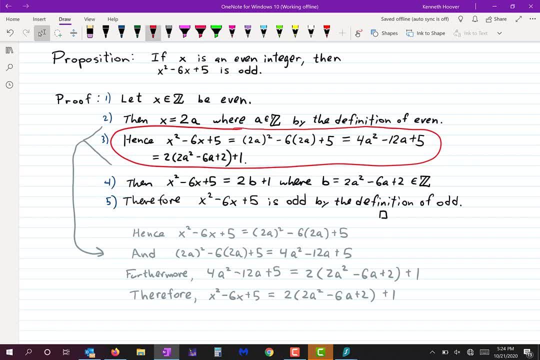 And that's the problem. The top part, that's written in red, that's one line that says these four lines. Okay, Now, just for the sake of- because I'm just trying to show you different ways you can do it, you could have done this. 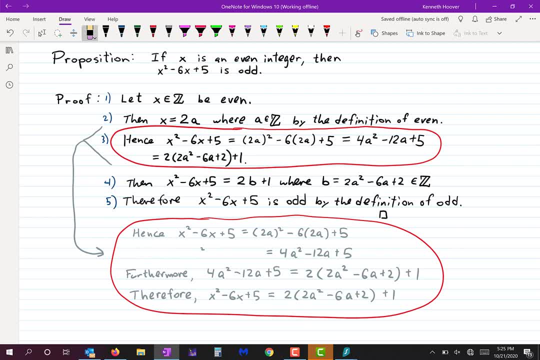 I could just erase everything before the equal signs, And that's it. And then this is literally the exact same thing as this. Look at it: It is identical, Just that, in order to save room going to the right, I just did a line break. Now, that is one long line. 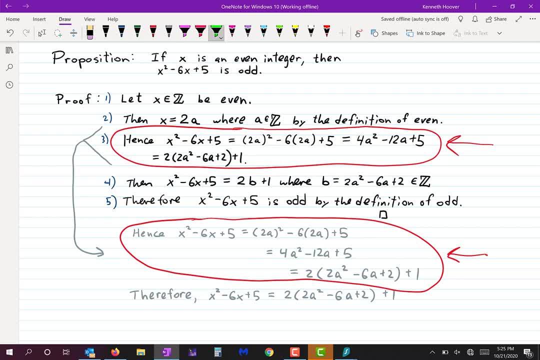 And because in that one line I have showed that this equals this. Now I no longer need this. You see how that is. If you learn this stuff that I'm trying to teach you here at the beginning, it's not that hard. So many people say. oh, proofs are so hard.